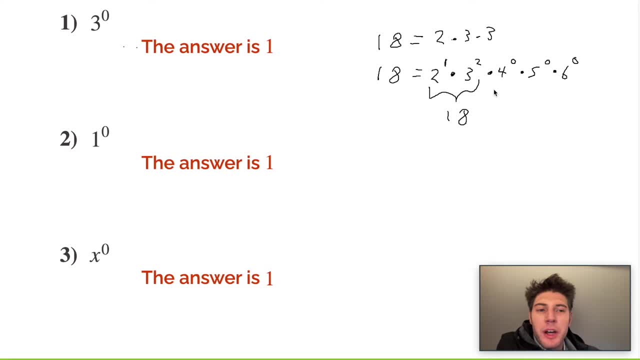 all need to be to leave us at 18?? Well, that would be 1.. So 4 to the 0 has to be 1.. 5 to the 0 has to be 1.. 6 to the 0 has to be 1.. So this isn't a proof or anything, but I thought it was kind of a. 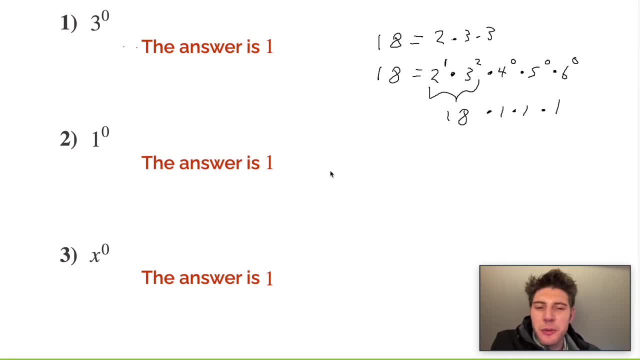 neat visualization for why it's 1.. I can show you another one. If you think of 2 squared, we can think of 2 cubed: 2 to the 4th, maybe 2 to the 1, and 2 to the 0.. So what is 2 squared? Well, that 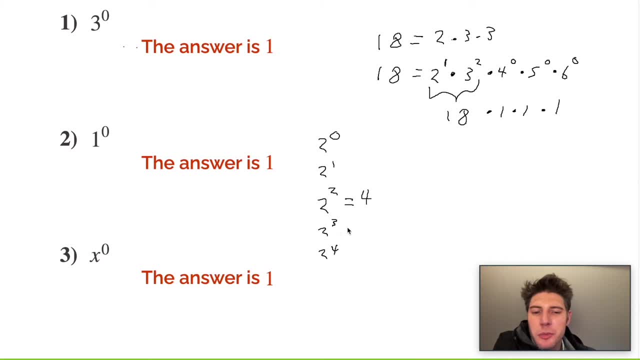 means 2 times 2,, so that's 4.. What's 2 cubed? Well, that's 2 times 2 times 2, so that's 8.. And 2 to the 4th would be 2 times 2 times 2 times 2, which is 16.. If we go up from here, we're dividing by 2. 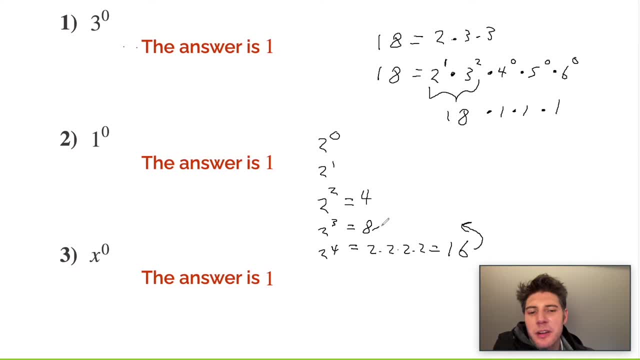 each time, 16 divided by 2 is 8.. 8 divided by 2 is 4.. 4 divided by 2 is 2.. And that makes sense, because we're dividing by 2 each time, So we're dividing by 2 each time, So we're dividing by 2. 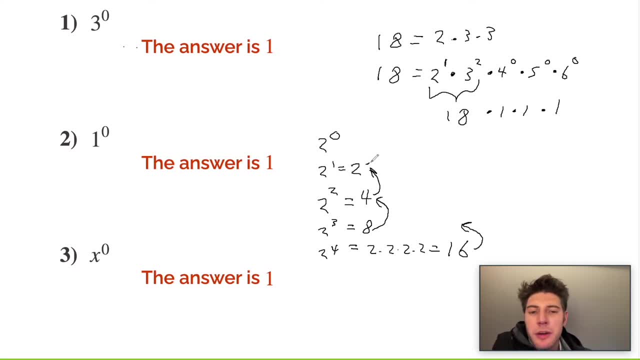 because 2 to the 1 would be 2.. And now, if we divide by 2 again, we get 1.. And look what that tells us: 2 to the 0 equals 1.. That's really interesting. Each of these times we just 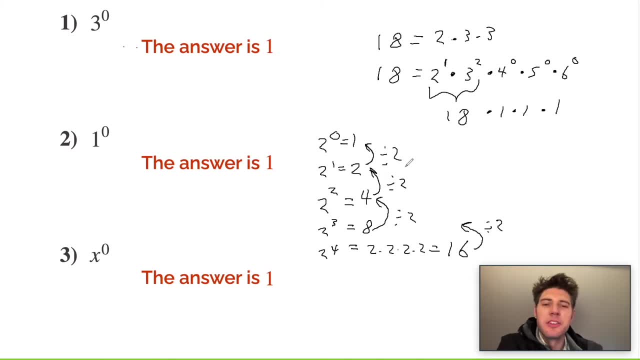 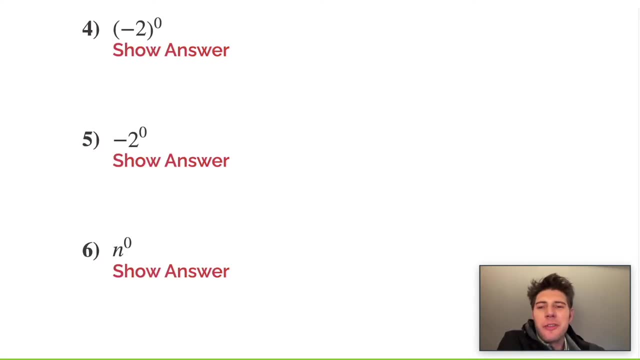 divide it by 2.. So once again, this isn't a proof, but these are just demonstrations of why a number to the 0 equals 1.. Let's try some more. So here are three more of these: Number 4, negative 2 to. 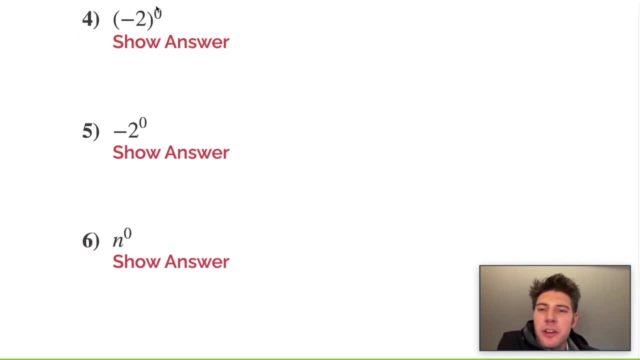 the 0. Well, since this is in parentheses, that means the 0 is going to the entire negative 2.. And we know that anything to the 0 equals 1.. So number 5 is very similar. I don't know if you noticed, but I really emphasized that this whole negative 2 was to the 0. The reason I 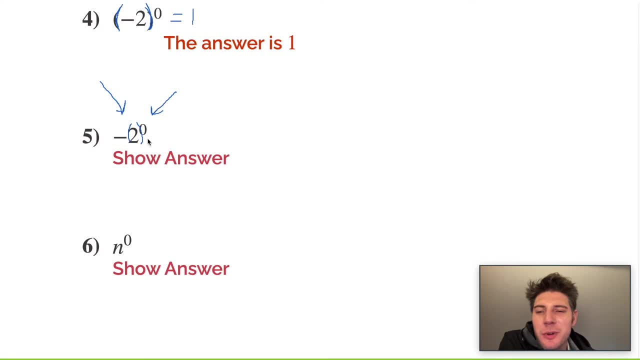 did, that is, in this problem only the 2 gets the 0 exponent. So that's all going to become 1.. But we still have this negative in front. So the answer to this one is negative 1.. And we can check it And the answer is negative 1.. The trick here is recognizing that unless there's a 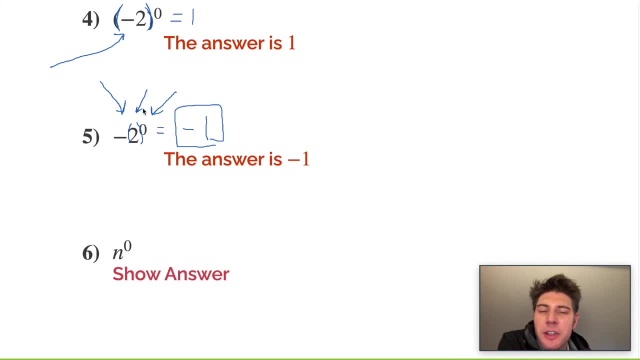 parentheses around it, the 0 exponent only goes to the number that it's touching. And then the answer of n to the 0, well, this is 1.. So we try some more. Let's do three more and then call it.